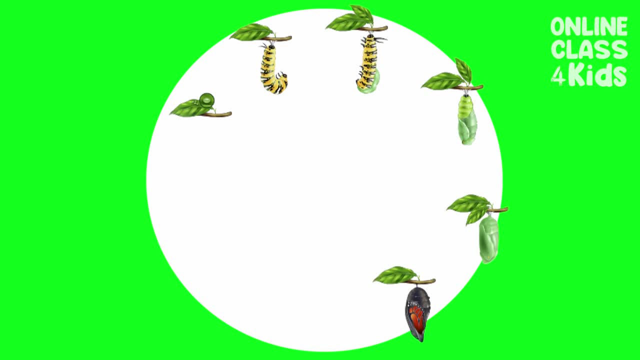 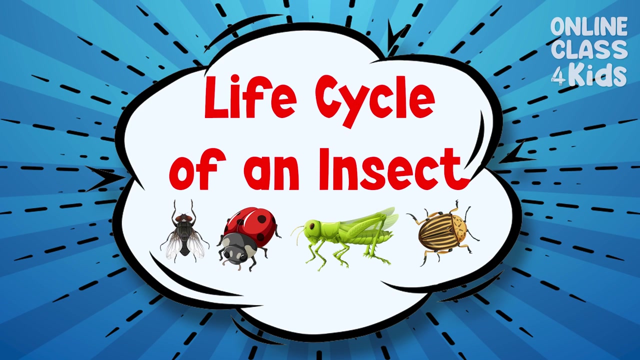 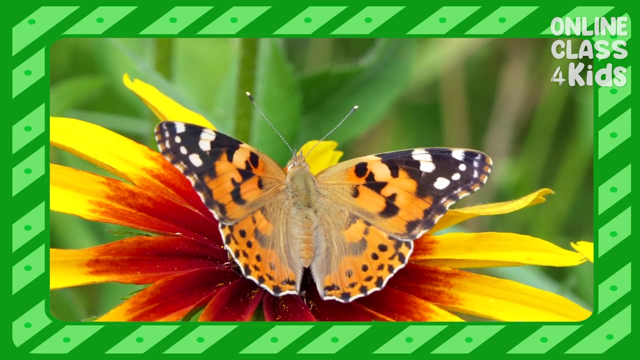 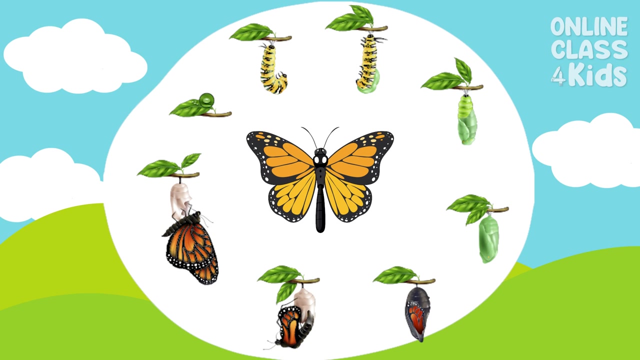 Unlike humans that give life birth, butterflies only lay eggs. Do you want me to tell you more about it? Alright, Let's discover About the life cycle, The life cycle of an insect. Let's have the butterfly as our example. The life cycle of an insect has four stages. 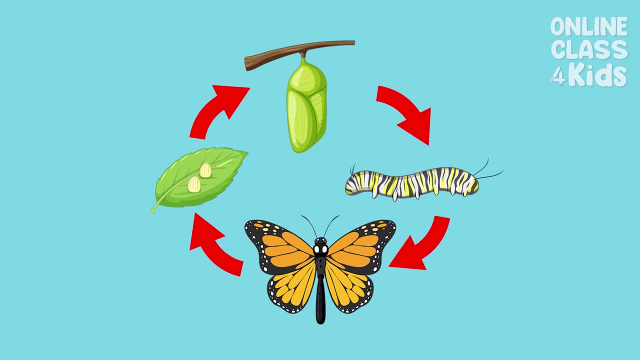 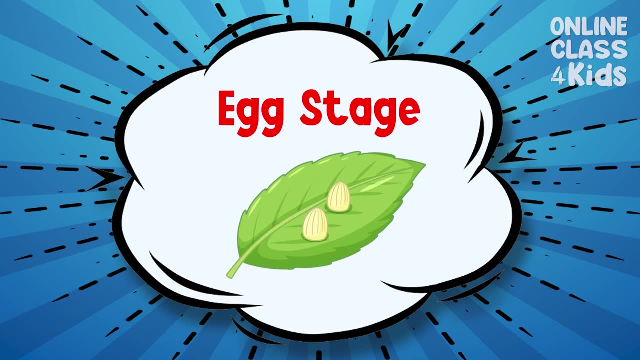 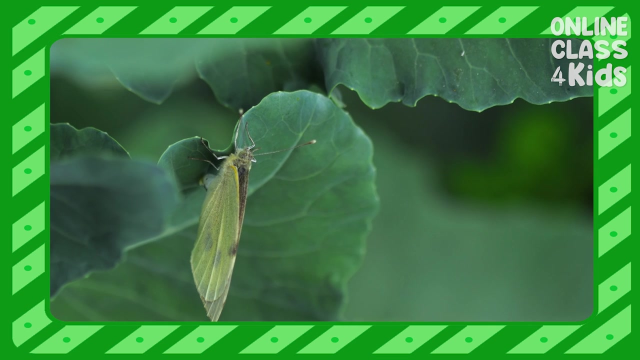 Let us learn about them one by one. Stage 1 is the egg stage. Insects begin their lives. They lay their first eggs. The duration of the egg stage can vary, but for a butterfly it usually lasts 3 to 7 days. 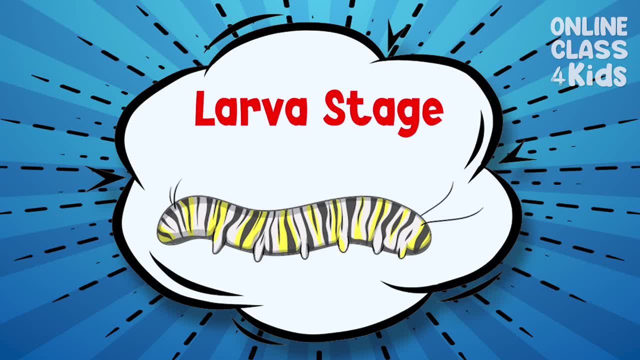 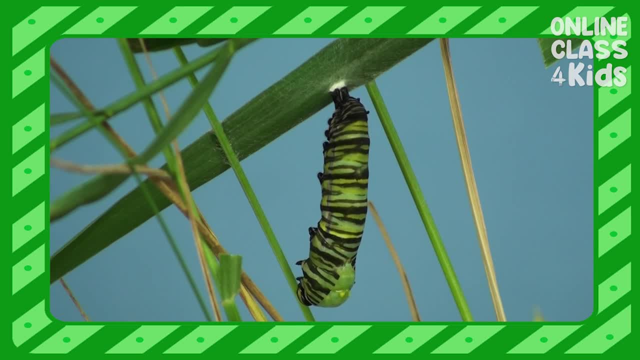 Stage 2 is the larva stage. This is where the eggs will hatch. A very tiny caterpillar hatches from a butterfly egg. They eat a lot of leaves. They eat a lot of leaves. They grow bigger. Stage 3 is the pupa stage. 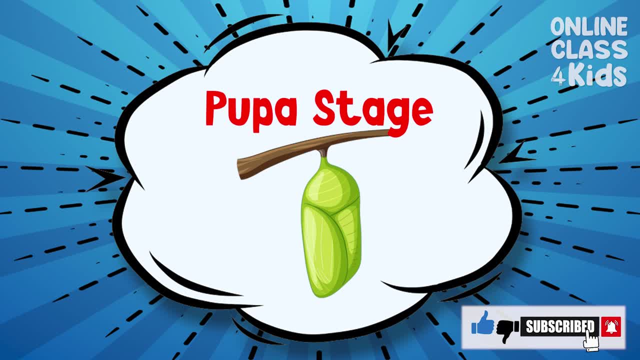 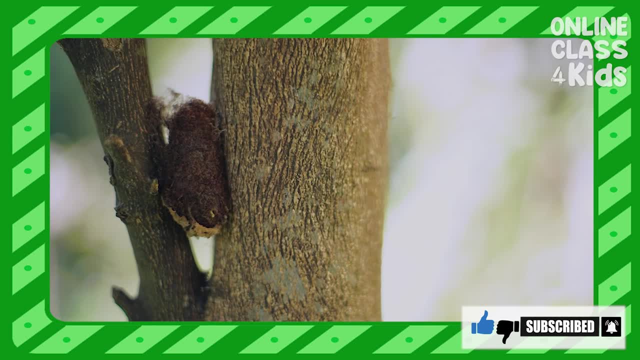 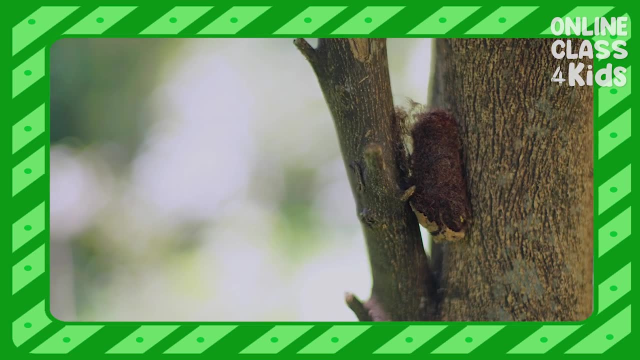 During this stage, the pupa is mostly resting and inactive. The wings of the insect are developed during this stage. This is also called the chrysalis stage for a butterfly. Stage 4 is the adult stage. It is the last stage of an insect's life cycle. 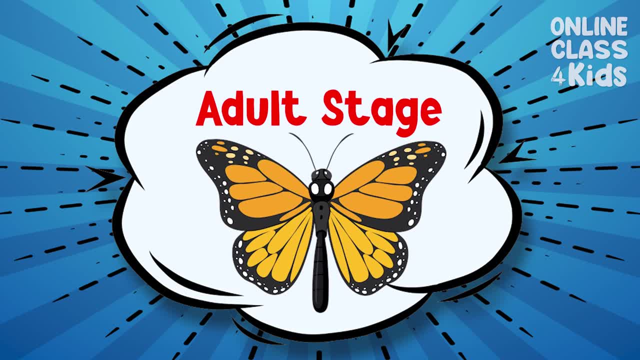 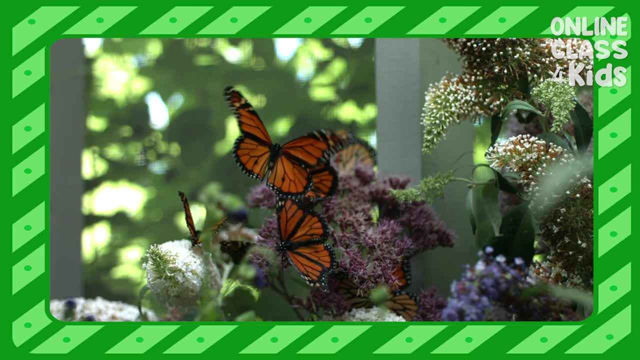 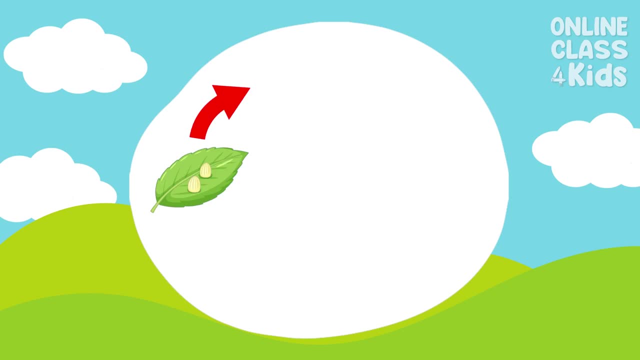 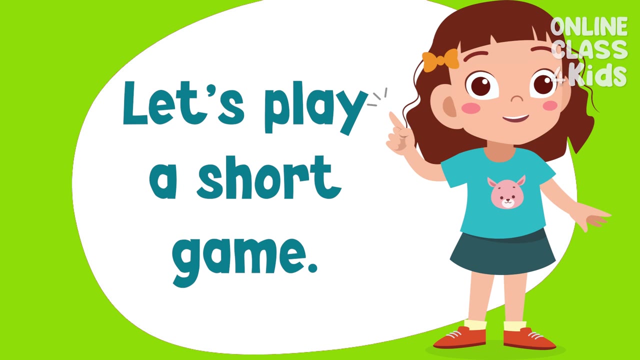 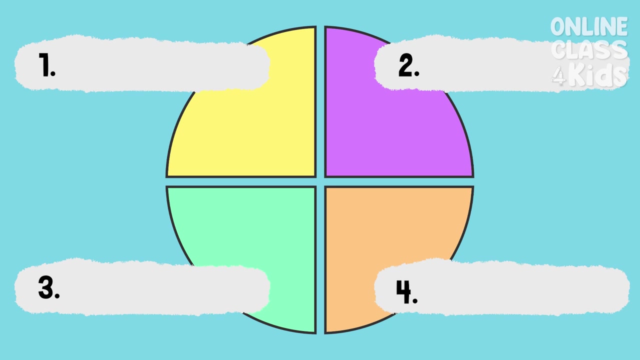 In this stage, the adult insect is mature and spends its time mostly reproducing to form another insect And the life cycle begins again. Let's play a short game. Let's complete the picture by answering some questions. Are you ready? Let's start. 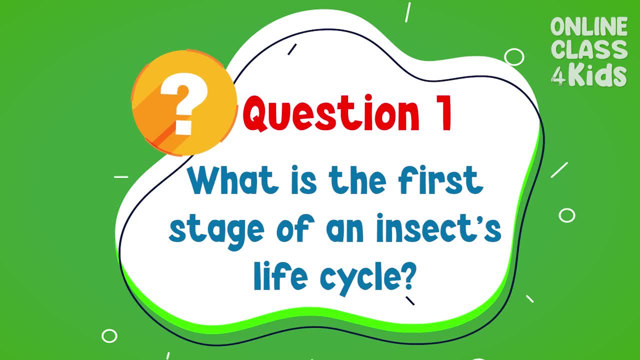 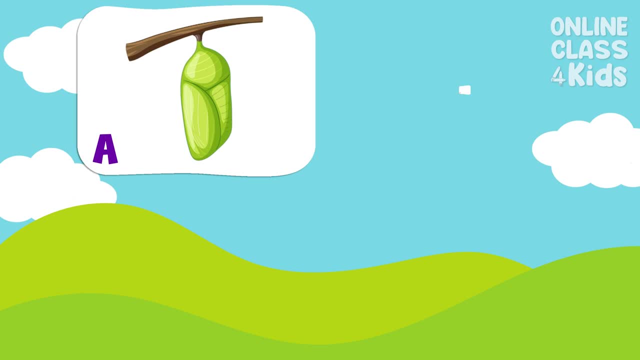 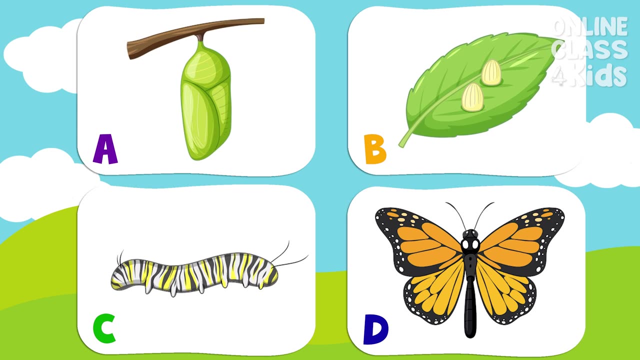 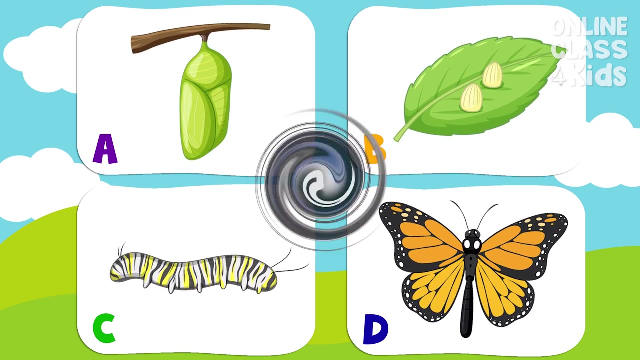 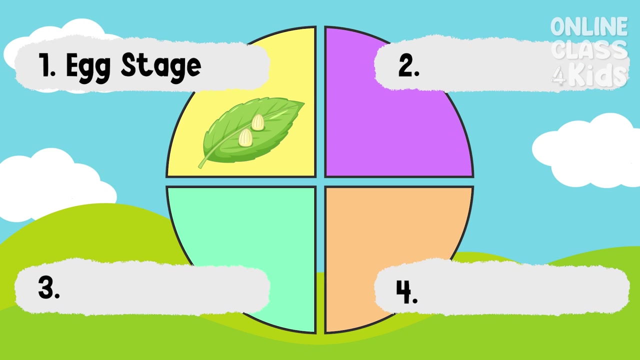 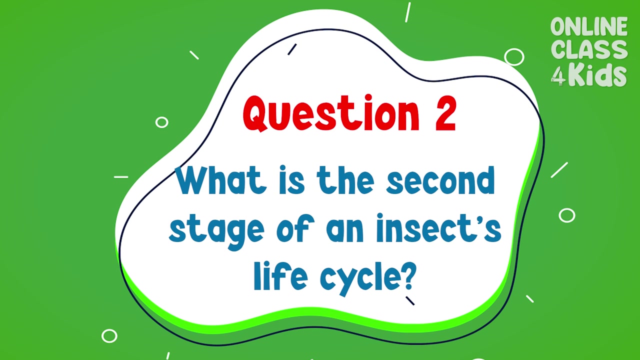 What is the first stage of an insect's life cycle? Is it A, B, C Or D Or D? Letter B: The first stage of an insect's life cycle is the egg stage, Very good. What is the second stage of an insect's life cycle? 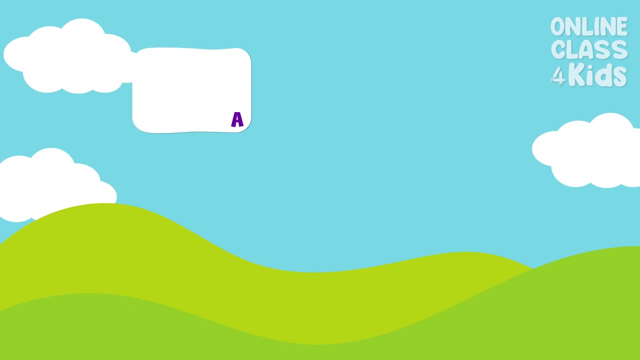 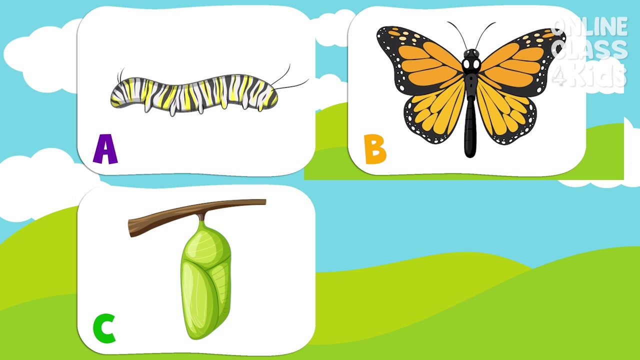 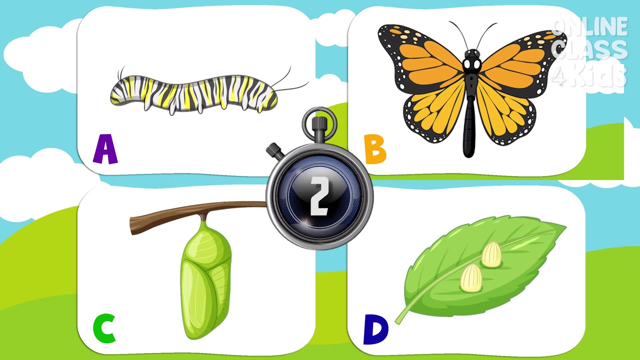 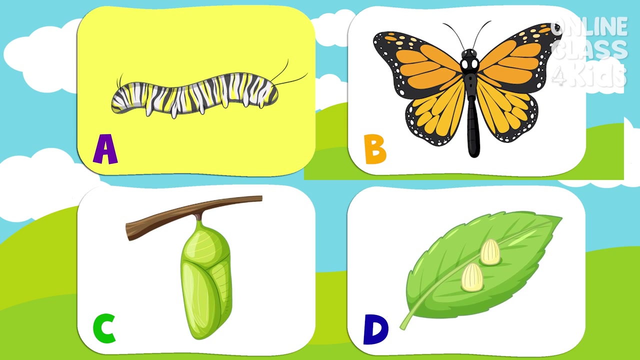 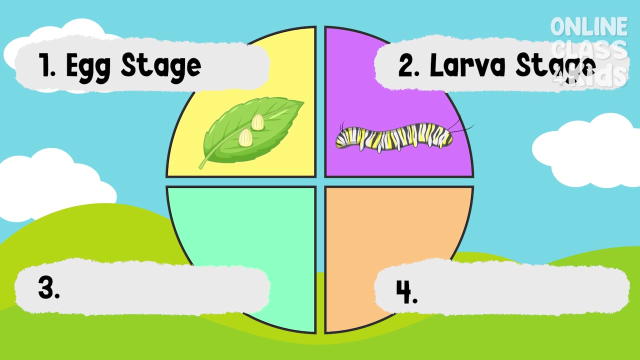 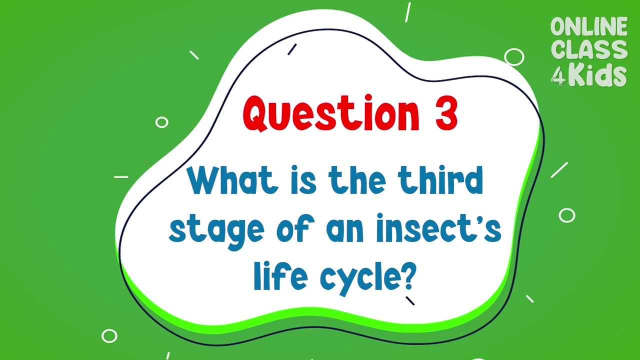 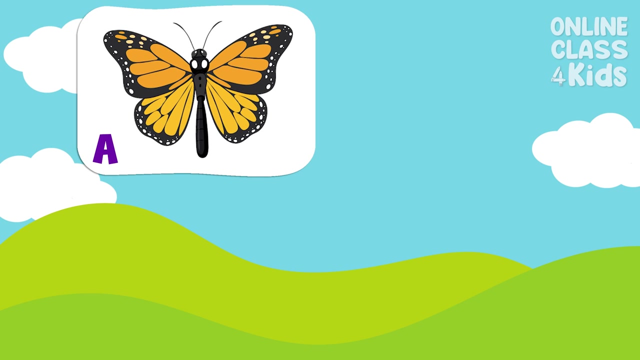 Is it A, B, C Or D? Letter A: The second stage of an insect's life cycle is the larvae. Very good. What is the third stage of an insect's life cycle? Is it A, B, C Or D? 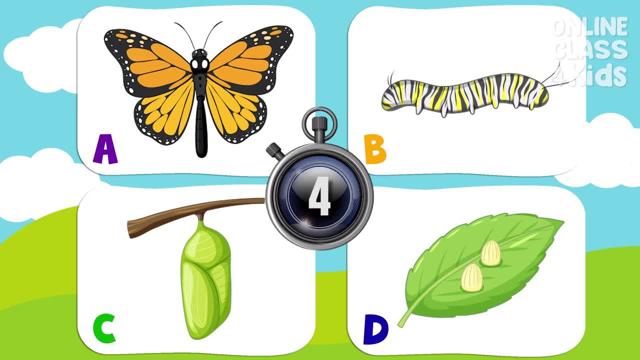 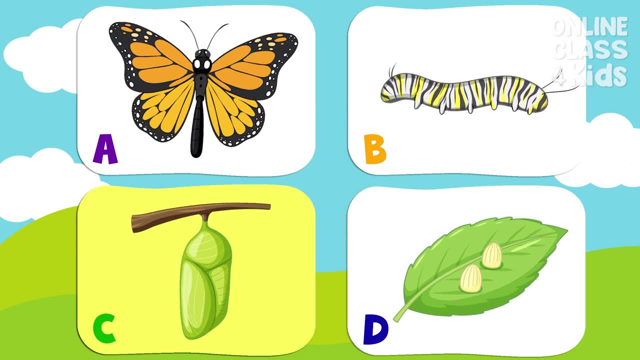 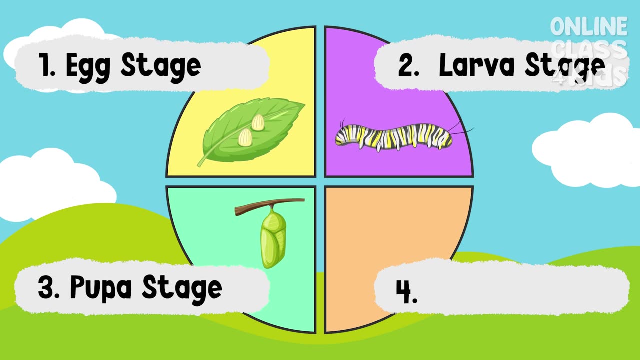 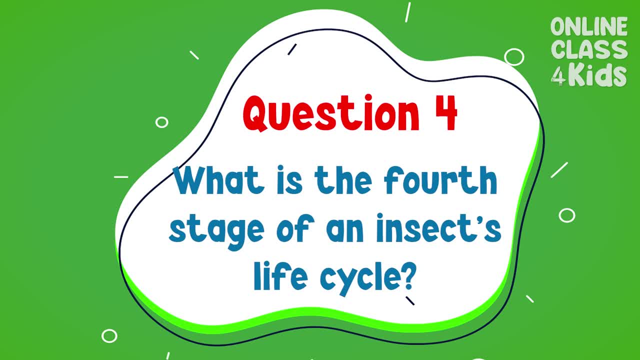 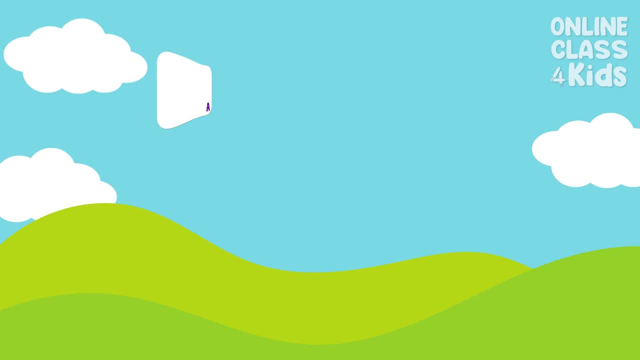 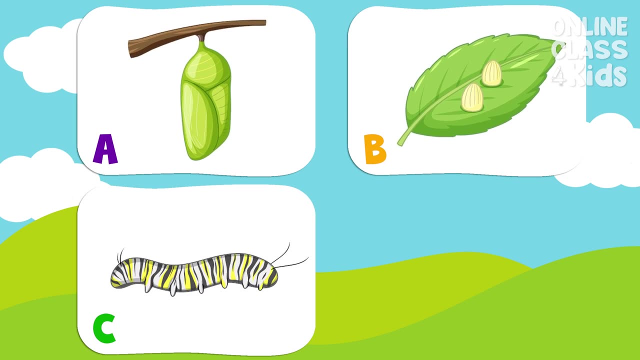 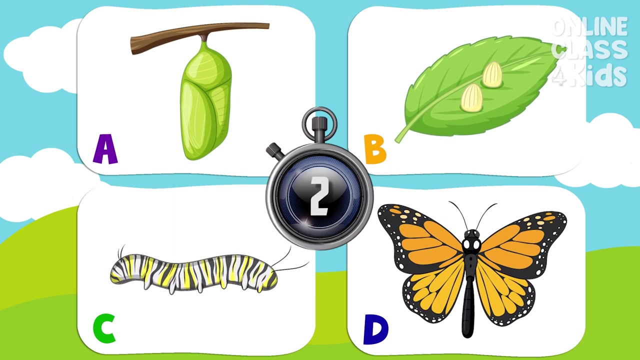 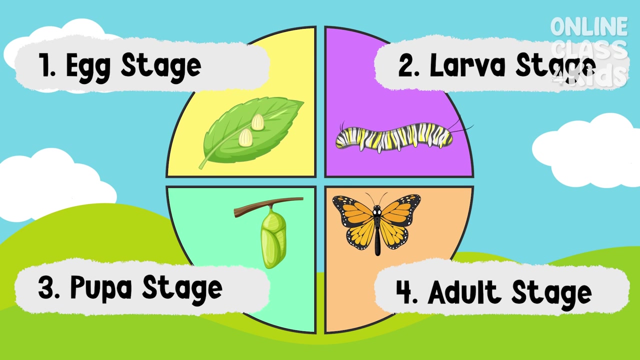 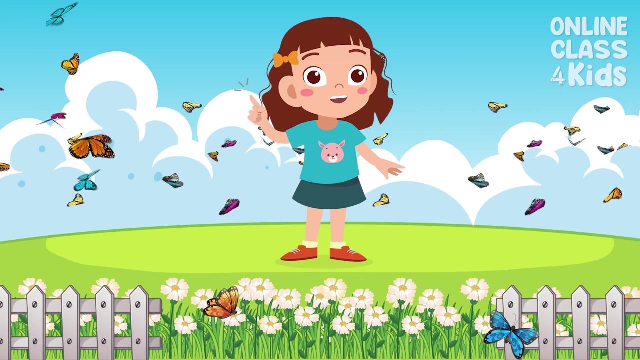 Very good. What is the first stage of an insect's life cycle? Is it A, B, C? The fourth stage of an insect's life cycle is the adult stage. Very good, You did great. I hope you had a wonderful time learning about the life cycle of an insect.